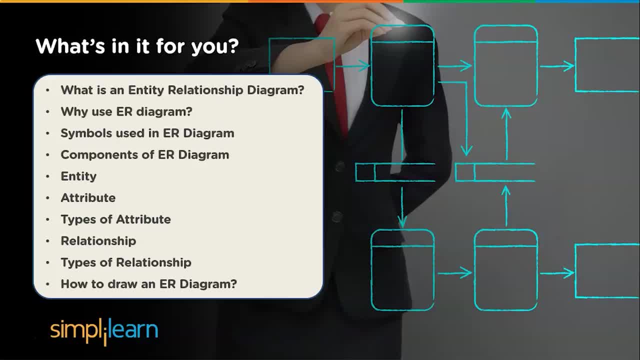 ER Diagram and get familiar with the components of it. So hey everyone, I am Abhisay Rawja from SimpliLearn and welcome to this video on ER Diagram in DBMS. But before we begin, if you love watching tech videos, subscribe to our channel and 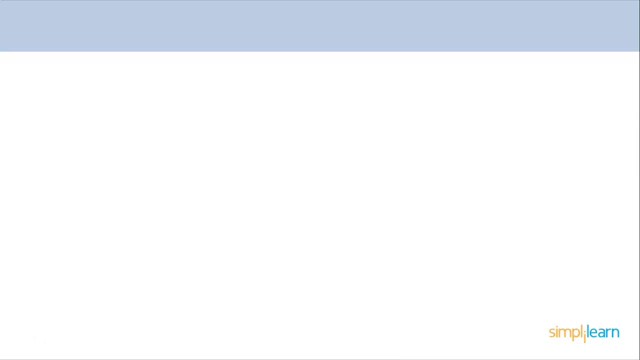 hit the bell icon to never miss an update. Let's start. Have you ever wondered how these big e-commerce companies manage their tons of data that keeps updating every second and these datasets keep on updating in their databases? to perform operations on this data, They should have a conceptual understanding of 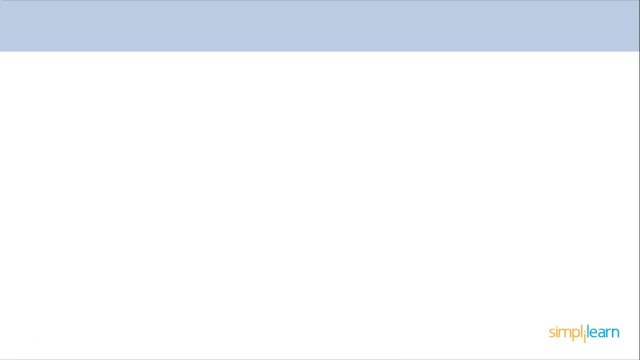 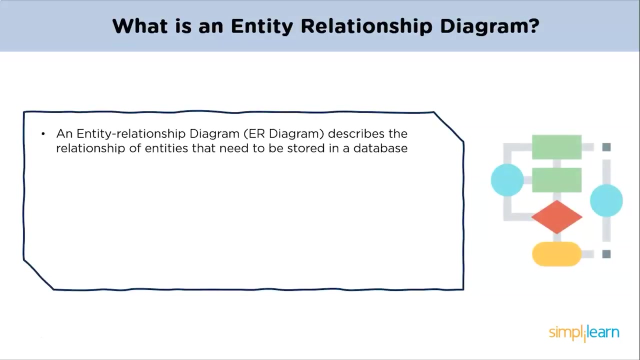 these databases and this is done by understanding ER diagrams of the databases. So let's understand what an ER diagram is. An entity relationship diagram describes the relationship of entities that needs to be stored in a database. ER diagram is mainly a structural design for the database. It is a framework made using specialized symbols to define the relationship. 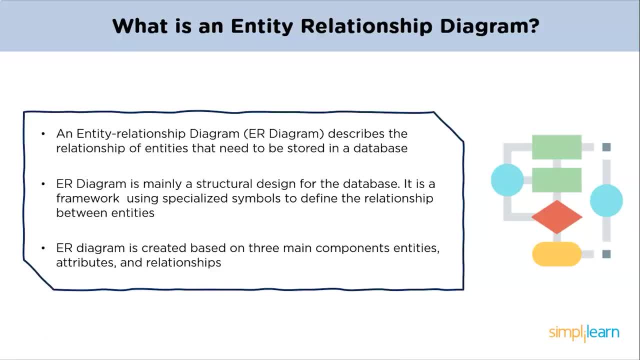 between entities. ER Diagrams are created based on the three main components: entities, attributes and relationships. Let's understand the use of ER Diagram with the help of a real-world example. Here, a school needs all its student records to be stored digitally. 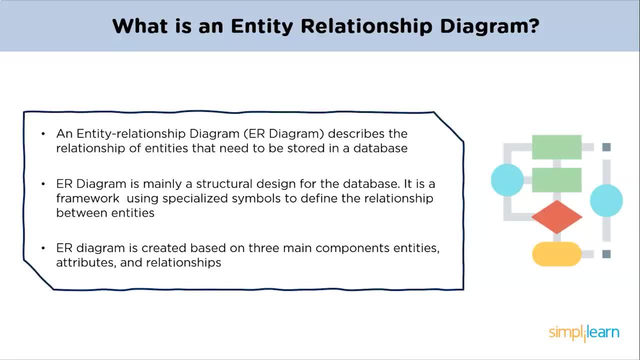 So they approach an IT company to do so. A person from the company will meet the school authorities, note all their requirements, describe them in the form of ER Diagram and get it cross-checked by the school authorities. As the school authorities approve the ER Diagram, the database engineers would carry further. 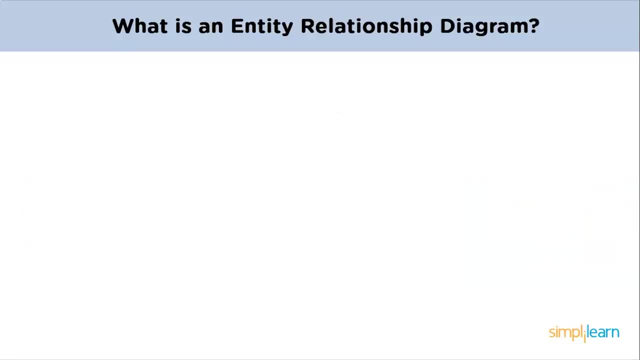 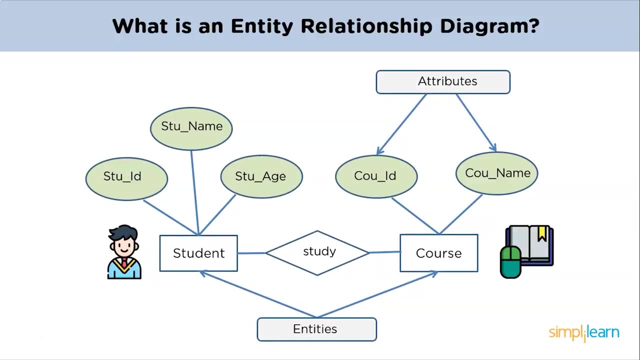 implementation. Let's have a view of an ER Diagram. The following diagram showcases two entities, student and course, and their relationship. The relationship described between student and course is many-to-many, as a course can be opted by several students And a student can opt for more than one course. 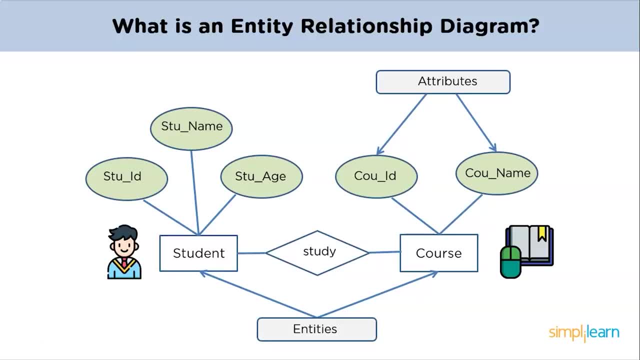 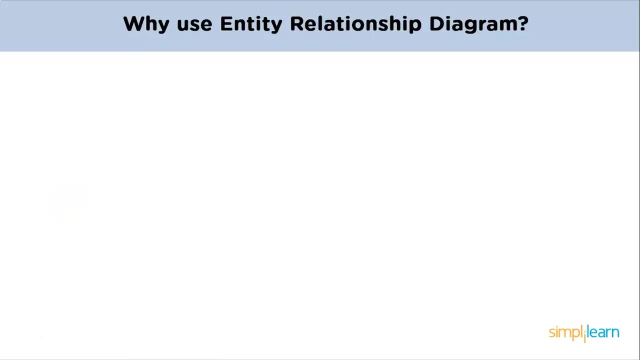 Here, student is the entity and it possesses the attributes, ie student ID, student name and student age, And the course entity has attributes such as course ID and course name. Now we have an understanding of ER Diagram. Let us see why it has been so popular. 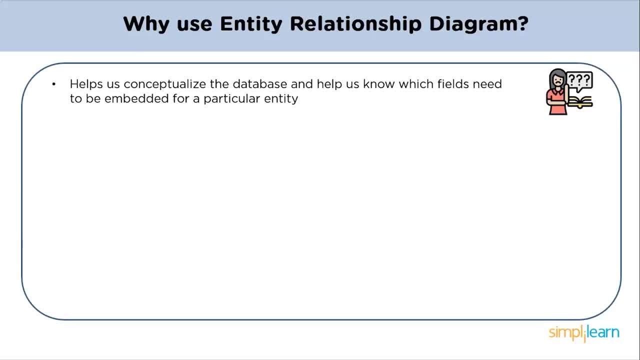 The logical structure of the database provided by ER Diagram communicates the landscape of business to different teams in the company, Which is why it is so popular. It is eventually needed to support the business. ER Diagram is a GUI representation of the logical structure of a database which gives 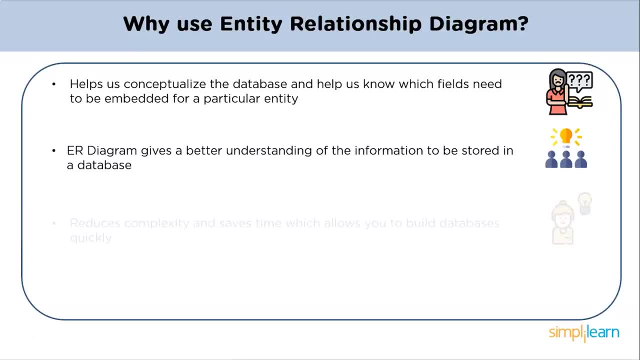 a better understanding of the information to be stored in a database. Database designers can use ER Diagrams as a blueprint, which reduces complexity and helps them save time to build databases quickly. ER Diagrams help you identify the entities that exist in a system and the relationships. 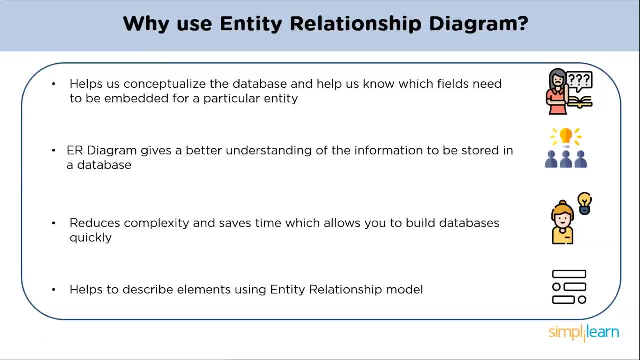 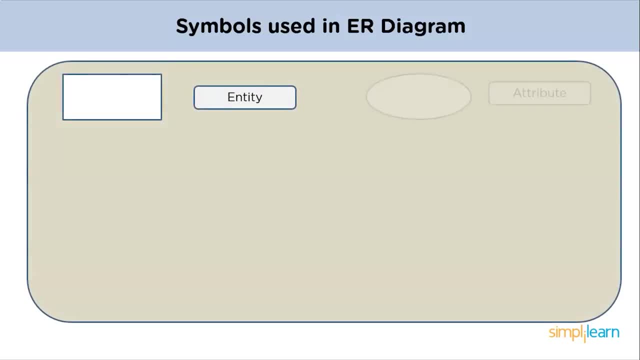 between those entities. After knowing its uses, now we should get familiar with the symbols used in ER Diagram. The rectangle symbol represents the entities. oval symbol represents attributes. a rectangle embedded in a rectangle represents a weak entity. a dashed oval represents a derived. 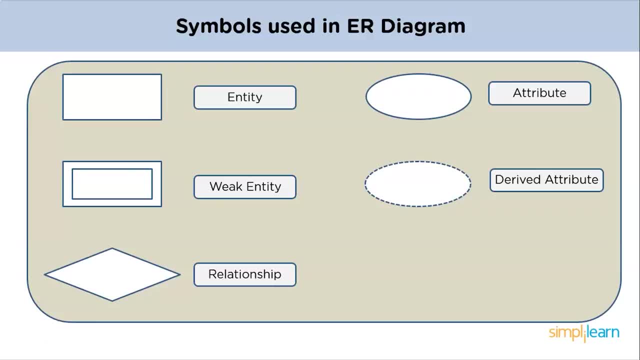 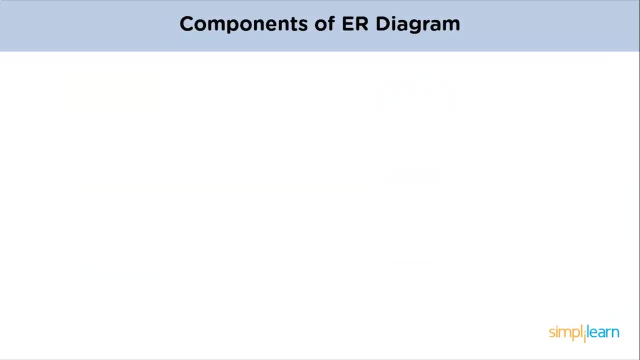 attribute. a diamond symbol represents a relationship among entities. double-oval symbol represents multi-valued attributes. Now we should dive in and learn about the components of ER Diagram. There are three main components of ER Diagram: 1., 2., 3.. 4., 5., 6., 7., 8., 9., 10., 20., 21., 22., 22., 23., 24., 25., 25., 26., 26.. 27. 27., 28., 28., 29., 30., 31., 32., 33., 34., 35., 36., 37., 38., 39., 40., 41.. 42., 42., 43., 43., 44., 44., 44., 45., 46., 47., 48., 49., 51., 52., 53., 53., 54.. 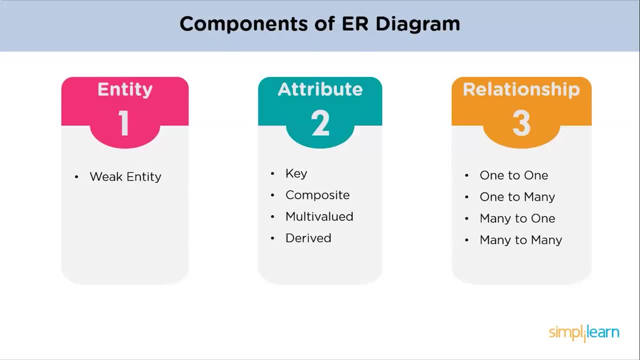 55., 56., 57., 57., 56., 57., 57., 58., 59., 59., 59., 60., 61., 61.. Let's understand these components of ER Diagram, starting with entities. 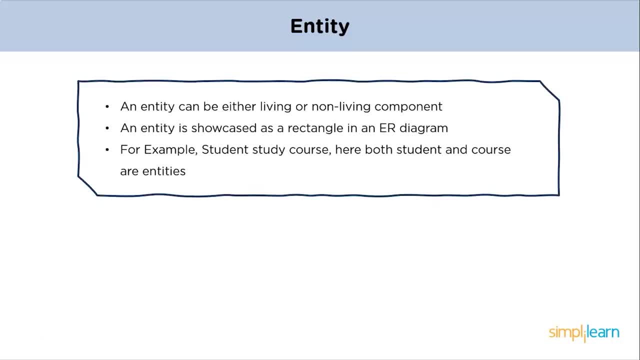 An entity can be either a living or a non-living component. An entity is showcased as a rectangle in an ER Diagram. Let's understand this with the help of an ER Diagram. Here, both student and course are in rectangular shape and are called entities. 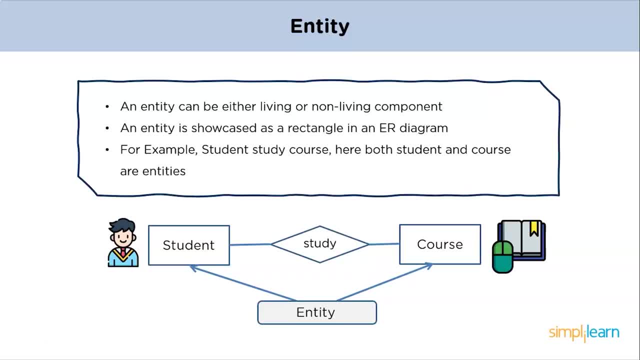 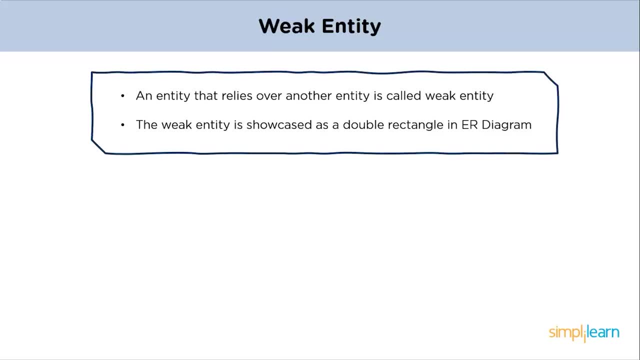 And they represent their relationship study in a diamond shape. Let's transition to weak entity. An entity that makes reliance over another entity is called a weak entity. A weak entity is showcased as a double rectangle in ER Diagram. In the example below, the school is a strong entity because it has a primary key attribute. 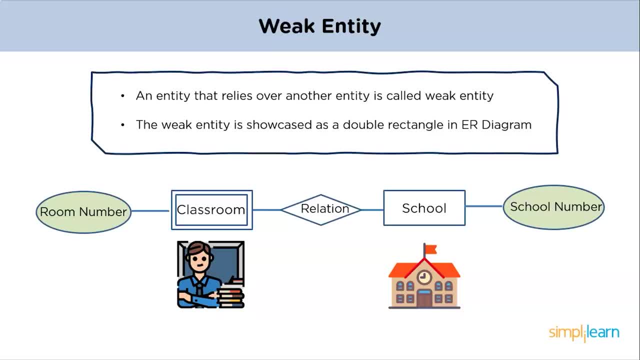 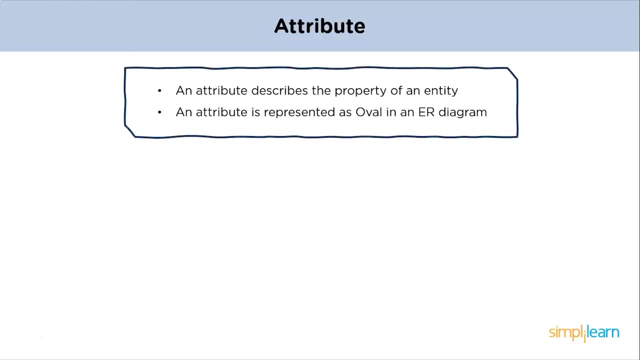 school number. Unlike the school, the classroom is a weak entity because it does not have any primary key, And the room number attribute here acts only as a discriminator and not a primary key. Now let us know about attributes. Attribute: An attribute exhibits the properties of an 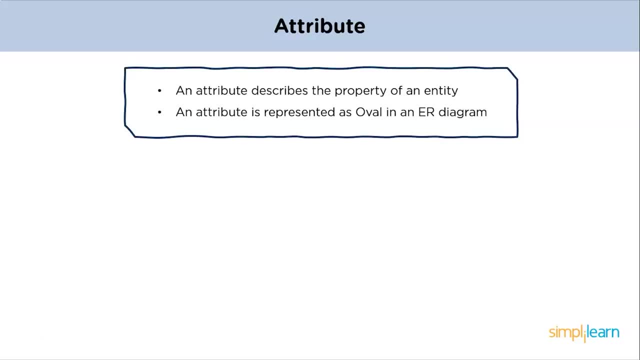 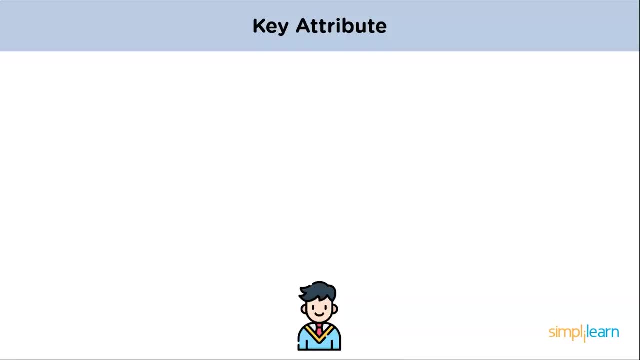 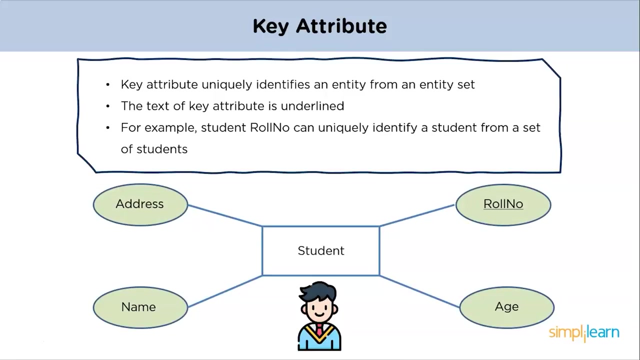 Let's see our first classification under Attribute, That is, Key Attribute. The key attribute uniquely identifies an entity from an entity set. The text of a key attribute is underlined In the example below. We have a student entity and it has attributes- name, address, role, number and age. but here 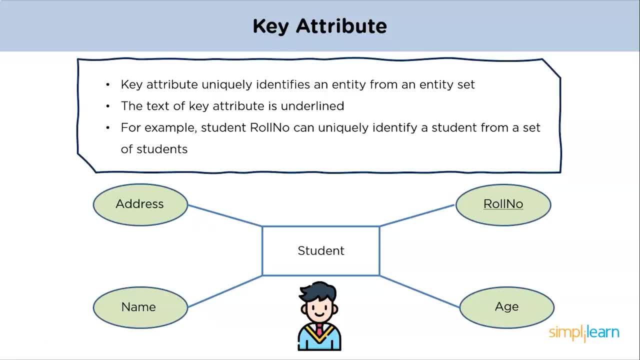 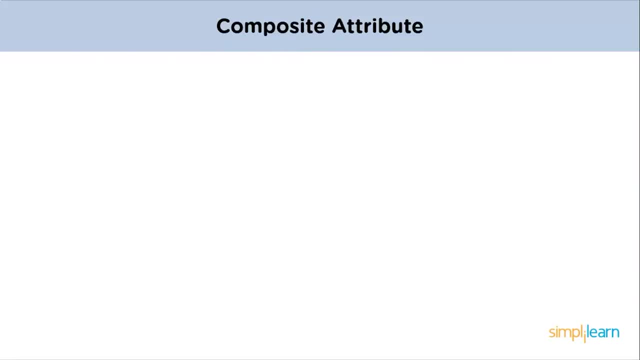 role number can uniquely identify a student from a set of students. That's why it is termed as a key attribute. Now we will see composite attribute. An attribute that is composed of several other attributes is known as a composite attribute. An oval showcases the composite attribute and the composite attribute. oval is further. 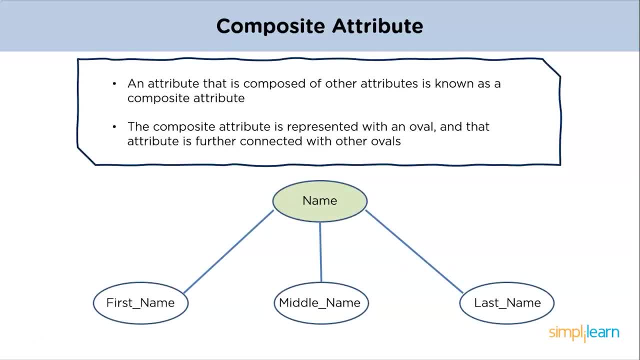 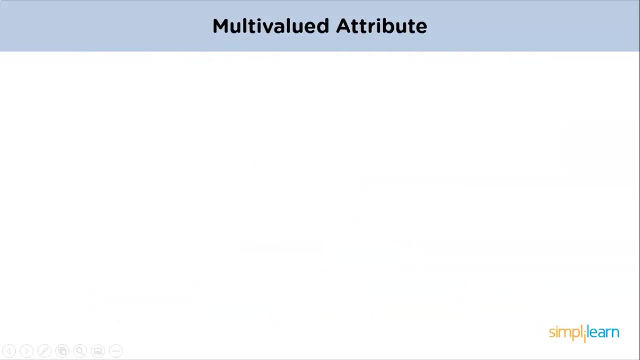 connected with other ovals. In the example below we can see an attribute name which can have further subparts, such as first name, middle name and last name. These attributes with further classification is known as composite attribute. Now let's have a look at multivalued attribute. 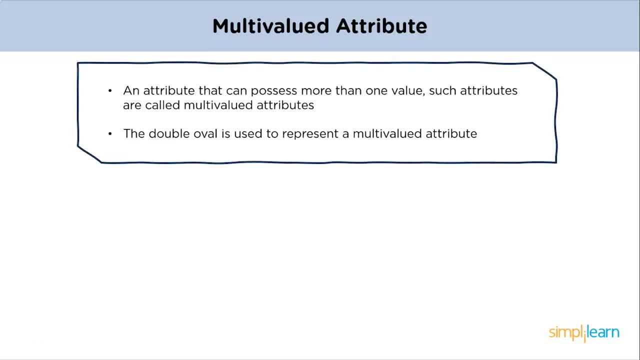 An attribute that can possess more than one value are called multivalued attributes. These are represented as double oval shape In the example below. the student entity has attributes phone number, role, number, name and age. Out of these attributes, phone number can have more than one entry and the attribute 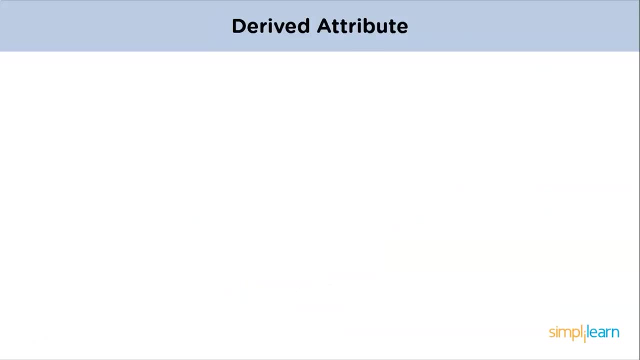 with more than one value is called multivalued attribute. Let's see derived attribute. An attribute that can be derived from other attributes of the entity is known as a derived attribute. In the ear diagram, The derived attribute is represented by dashed oval. 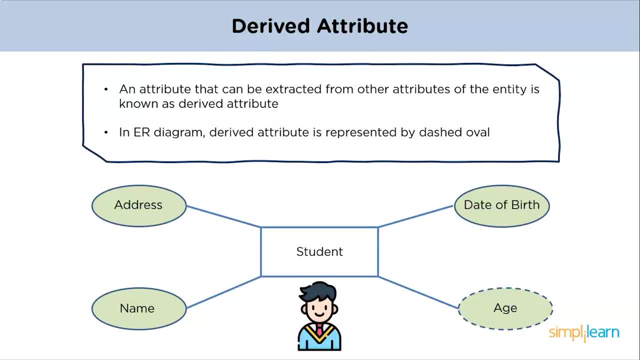 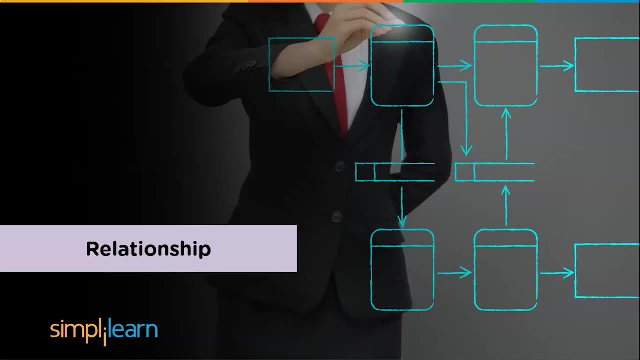 And in the example below, student entity has both date of birth and age as attributes. Here, age is a derived attribute, as it can be derived by subtracting current date from the student date of birth. Now, after knowing attributes, let's understand relationship in ear diagram. 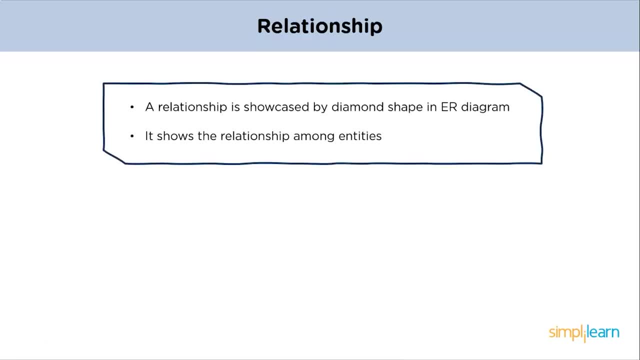 A relationship is showcased by the diamond shape in the ear diagram. It depicts the relationship between two entities In the below example: student study course. Here both student and course are entities and study is the relationship between them. Now let's go through the type of relationship. 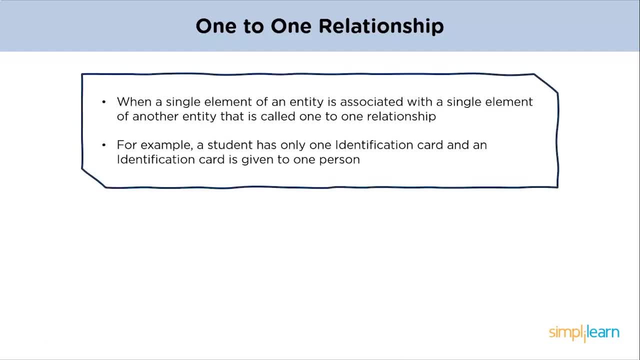 First is 1 to 1 relationship. When a single element of an entity is associated with a single element of another entity, This is called 1 to 1 relationship. In the example below we have student and identification card as entities. We can see a student has only one identification card and an identification card is given to 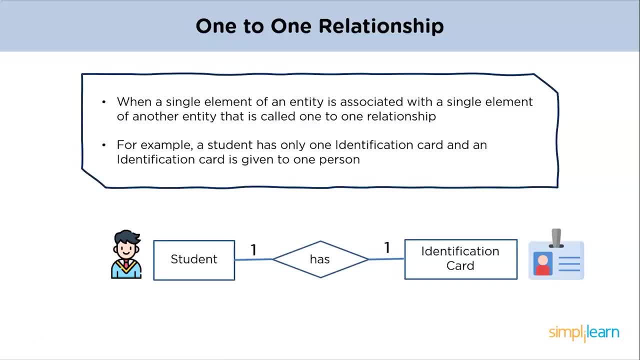 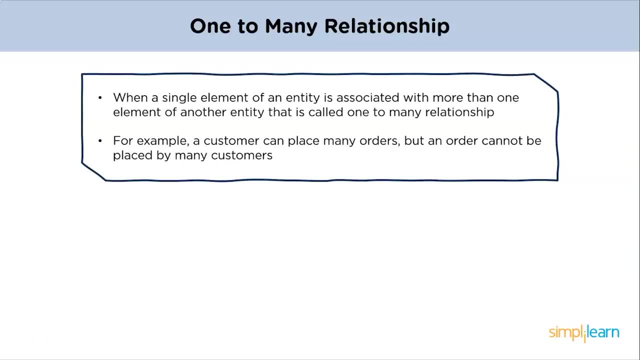 one student. It represents a 1 to 1 relationship. Let's see the second one: 1 to many relationship: When a single element of an entity is associated with more than one element of another entity is called 1 to many relationship. 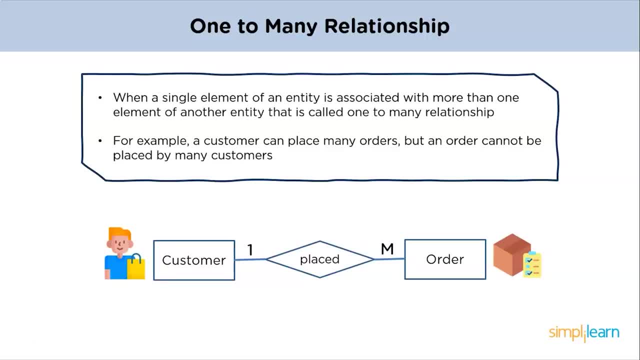 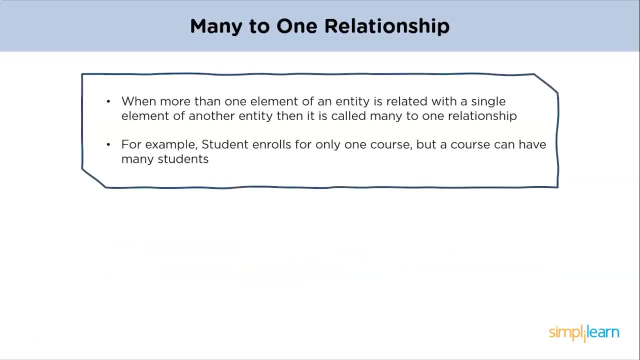 In the below example: a customer can place many orders, but a particular order cannot be placed by many customers. Now we will see the second one. 1 to many relationship: When more than one element of an entity is related to a single element of another entity. 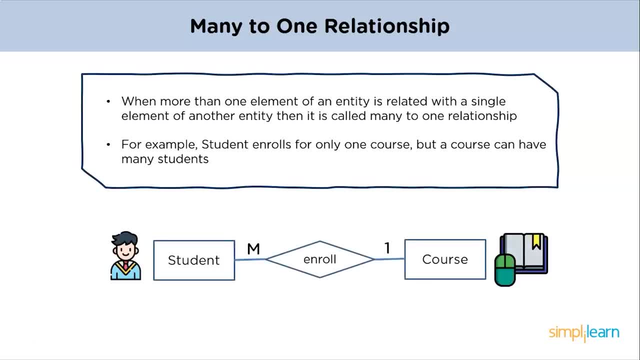 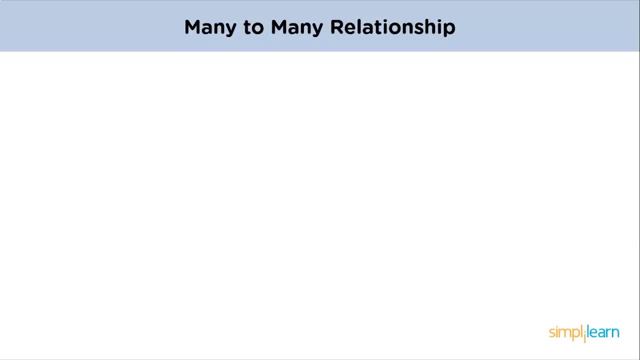 It is called 1 to many relationship. For example, students have to opt for a single course, but a course can be opted by number of students. Let's see 1 to many relationship When more than one element of an entity is associated with more than one element of another. 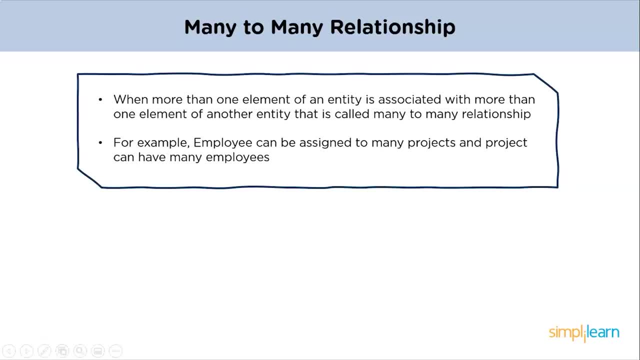 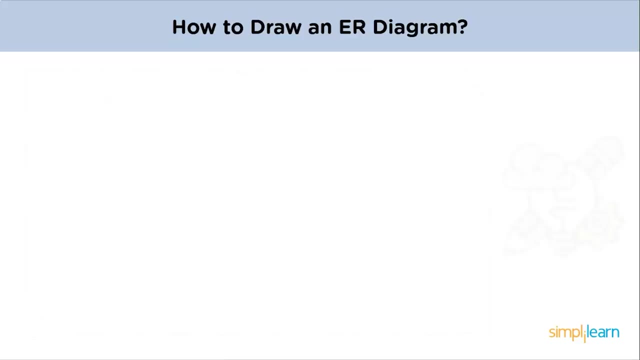 entity is called 1 to many relationship. For example, an employee can be assigned to many projects and many employees can be assigned to a particular project. Now, after having an understanding of the year diagram, let us know the points to keep in mind while creating the year diagram. 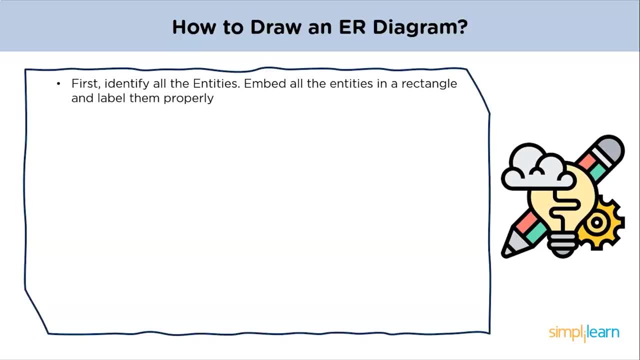 First, identify all the entities in the system. embed all the entities in a rectangular shape and label them appropriately. This could be a customer, a manager, an order, an invoice, a schedule, etc. Identify relationships between entities. For example, an employee can be assigned to many projects and many employees can be assigned.